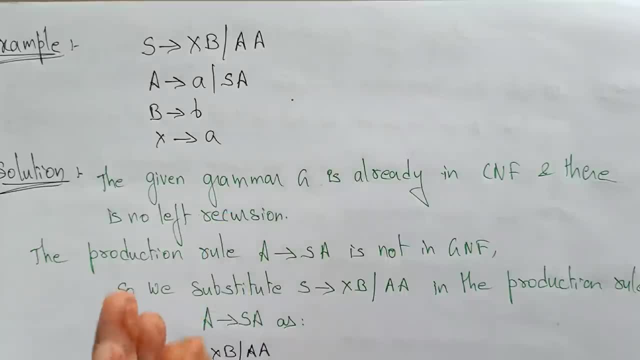 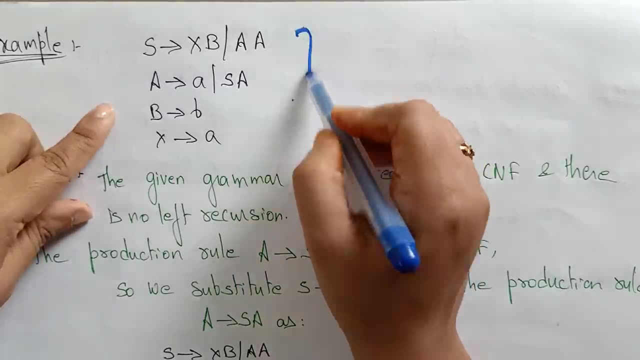 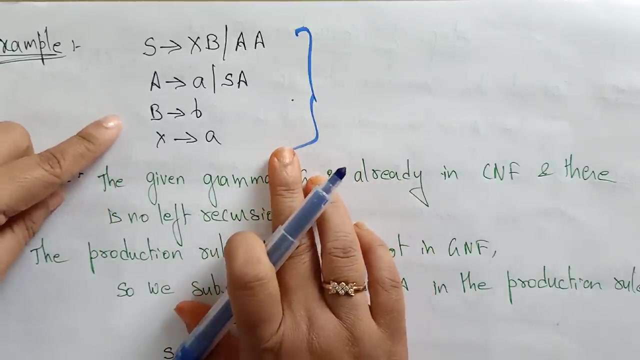 So don't confuse. Let's concentrate on this because this is somewhat a little confusion topic, So don't be confused and please keep concentrated here. So this is a grammar given, context-free grammar they are given. So first we need to check whether this grammar is in CNF or 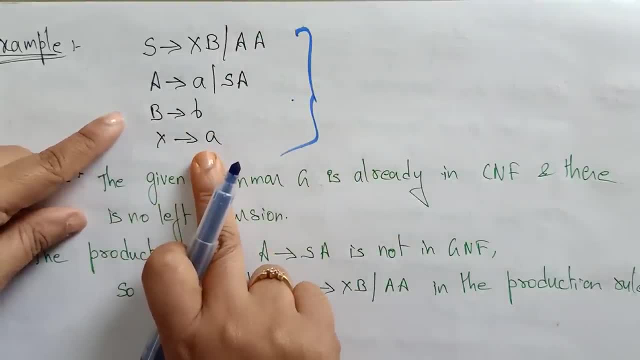 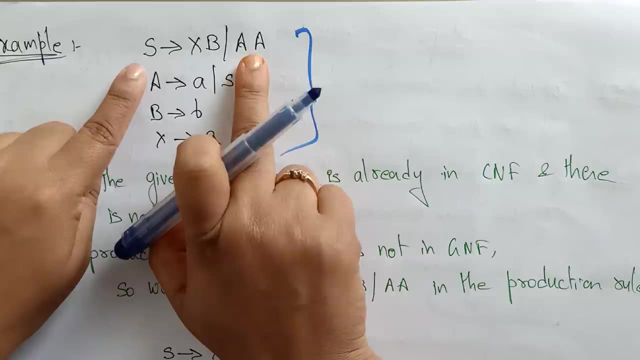 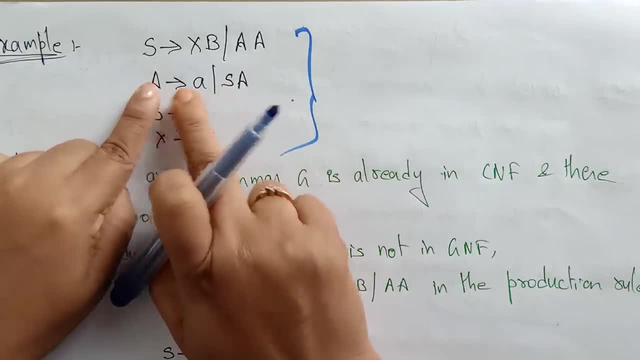 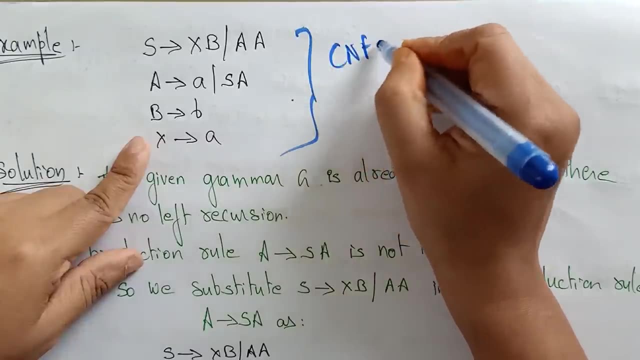 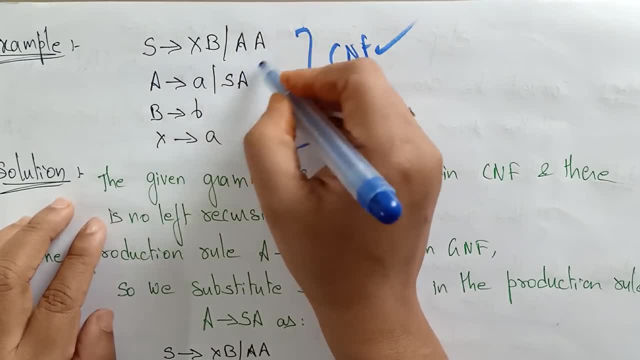 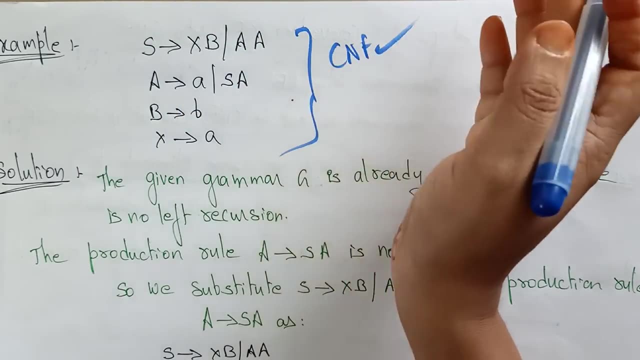 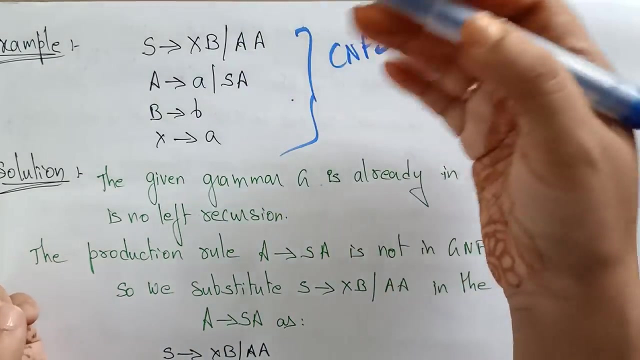 form And there is no left recursion also because it's only each non-terminal is generating. it's only two non-terminals, not more than that. If it is more than that- see three, two, and it is non-terminals, also repeating- then you can say it is a left. recursion is there, but here there is no left. 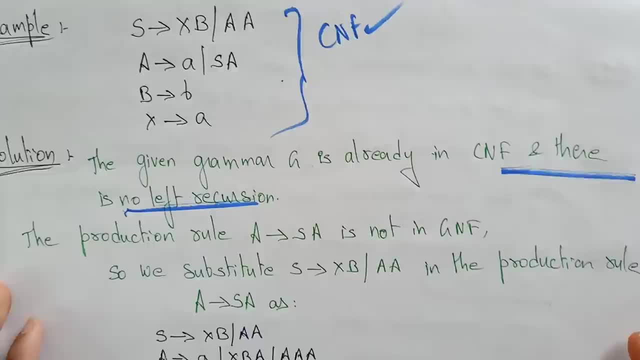 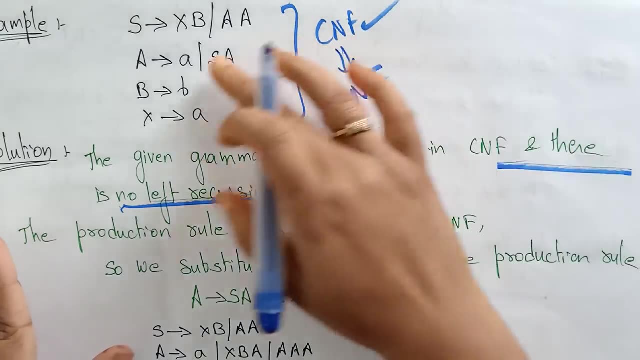 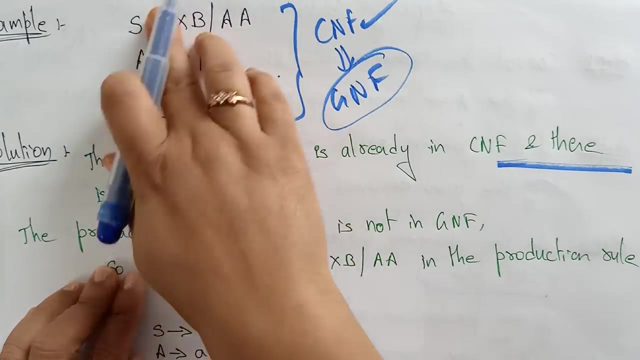 recursion also, so directly you can enter into the step. now i want to convert this cnf, the contact chomsky normal form into whatever the given context, free grammar, into greeback normal form. now let's see the first step. i can clearly say this is not in greeback normal form, why i can say: 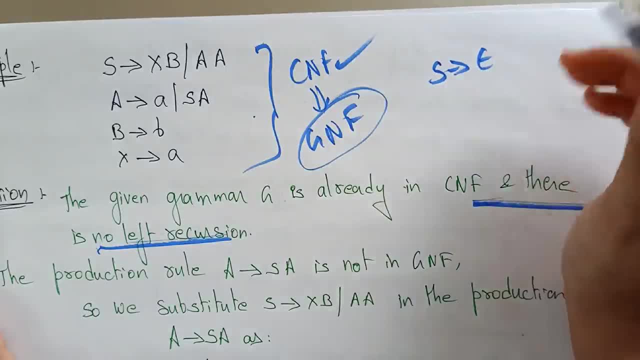 because the step says the start symbol has to generate epsilon or a terminal non-terminal. is generating a terminal or a non-terminal? the starting symbol should be a terminal, followed with any number of any number of non-terminals. so that is a condition. okay, so either it has to be. 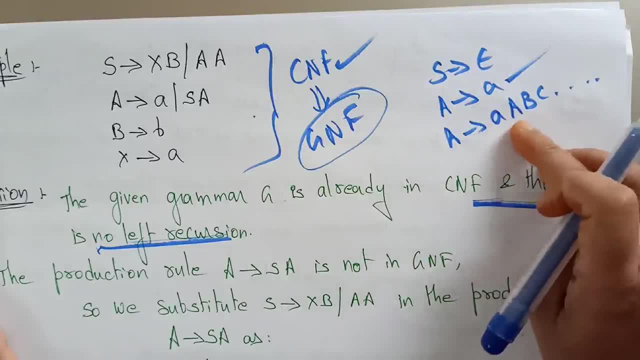 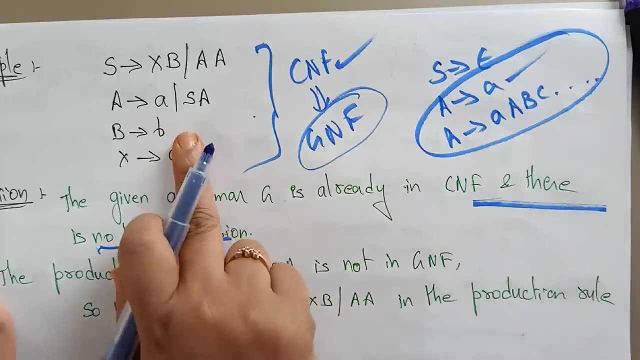 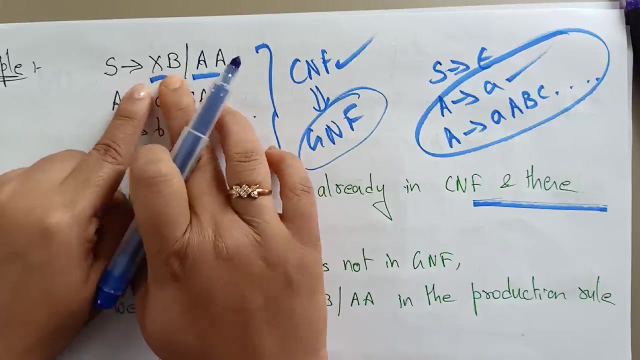 a single terminal, or it has to be single terminal followed with any number of non-terminals. so this is a condition for the gnf, the greeback normal form. but here it is violating the condition. see, here there is no terminal before that. uh, these two non-terminals. so this is in gnf only, but this: 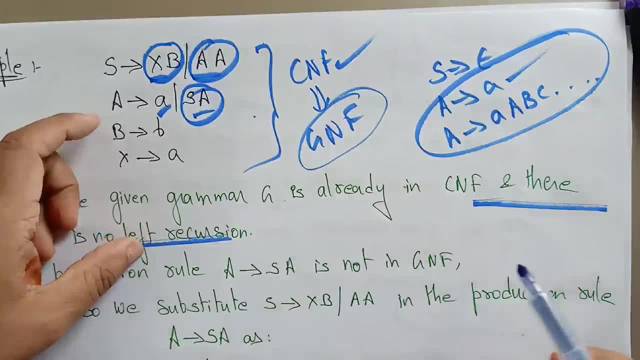 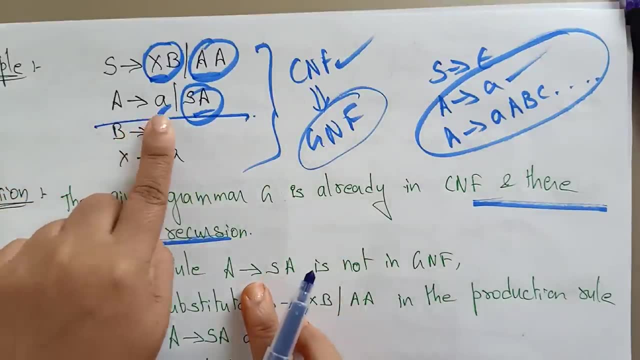 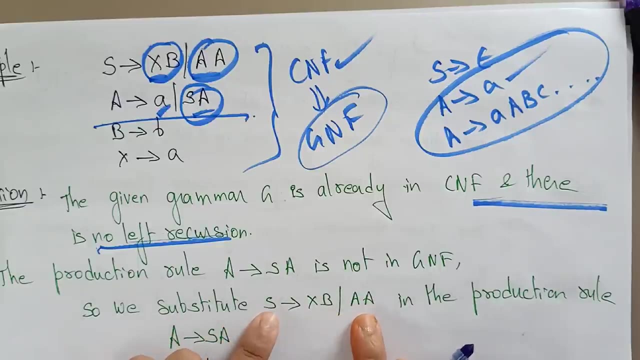 is not in gnf. so these three terms are not in productions are not in gnf. see here the production rule. first talk about this. a production rule: a determines sa is not in gnf. okay, so we substitute s determines xb or a in the production rule. so first i want to replace the start symbol with 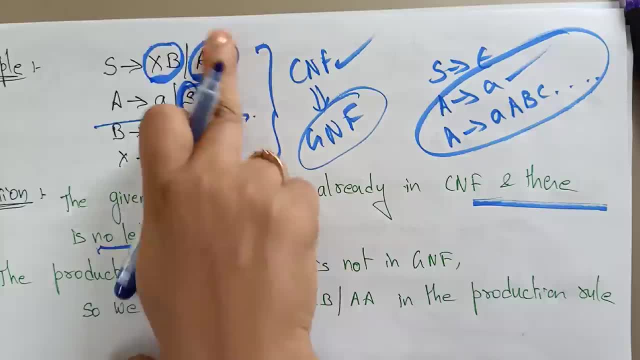 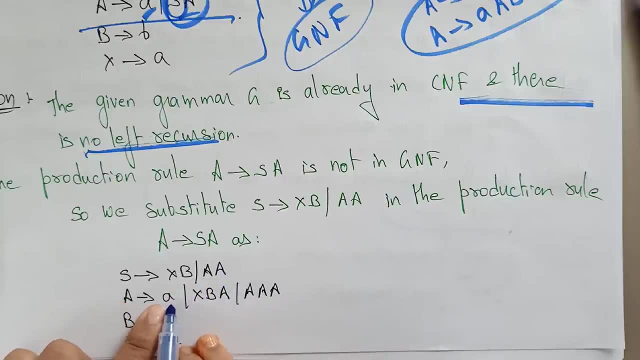 the productions. so just replace wherever the s here with this productions. okay, i replaced it. so this is s determines xb or aa, a determines a. so in place of sa, i'm writing: what is this xb? the first one is xb multiply a. or next production is aa. 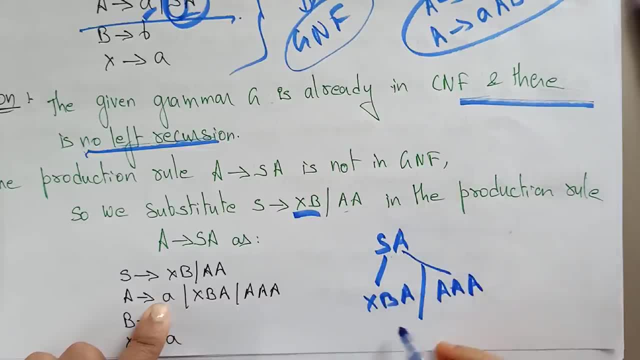 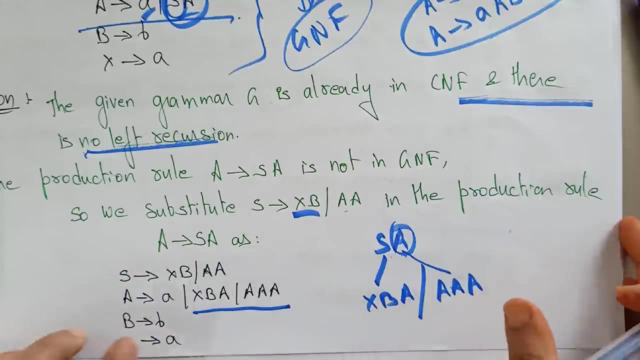 aa and this a has to be added, so this a should be multiplied with this production as well as this production. so this is my new production. i got, okay, b, b as it is. now let's again check: is this in gnf? no, it is not in gnf. again, this is having a left recursion also. all right, let me check. 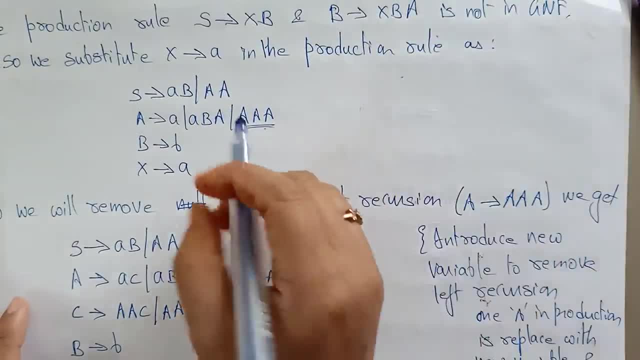 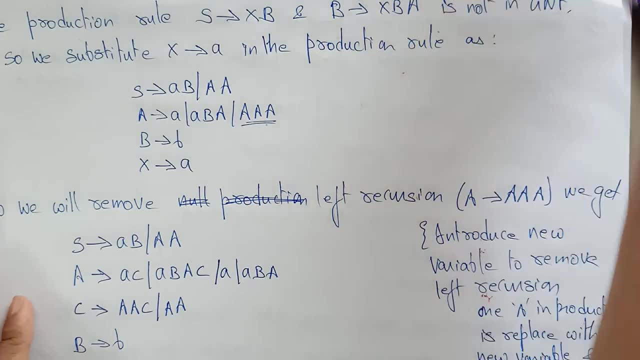 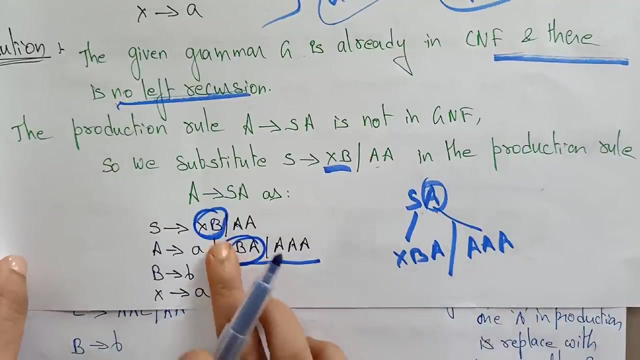 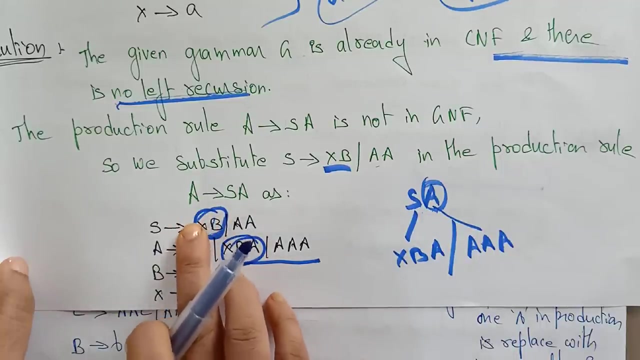 see here the production rule s determines xb and b determines xba. did you check here? so, before going to left, recursion s determines xb and a determines xba is also not in gnf, because the start symbol of this production should be: that is the right hand side, that is the first. 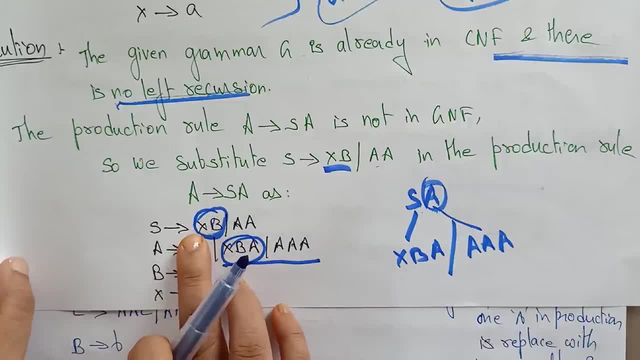 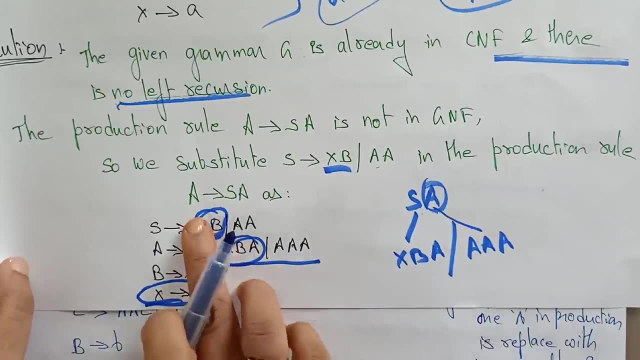 symbol of this production, not start symbol. the first symbol of this production should be a terminal should be there. so i am just replacing x determine a in place of x. then i will get my gnf right. okay, see here the production rule on x is not in gnf. so before going to left recursion, let's check here. s determines xb and a. 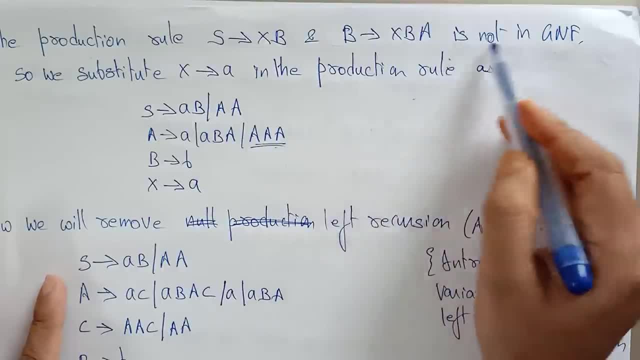 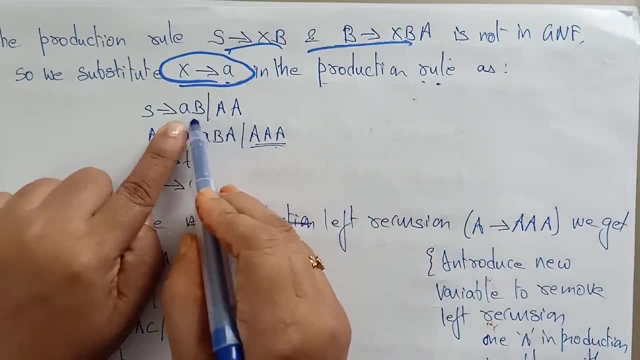 S determines XB and B determines XBA is not in GNF. So I am substituting X, determine A in the production rule. Now I substituted In place of X, I substituted A. Now this is in GNF. This is. 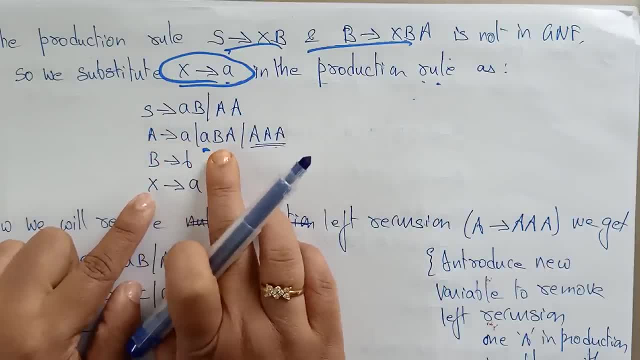 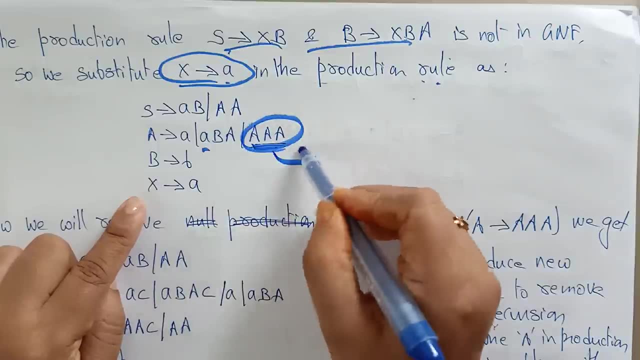 in GNF, GNF, GNF, GNF, because a terminal is followed with non-terminals. Now, these are all in GNF, Only these two are not in GNF. But it is a left recursion. It is providing a left recursion. 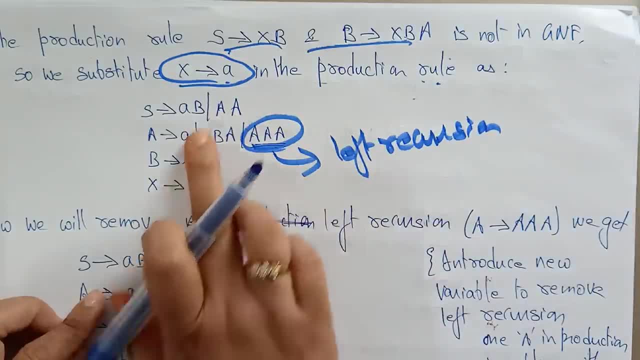 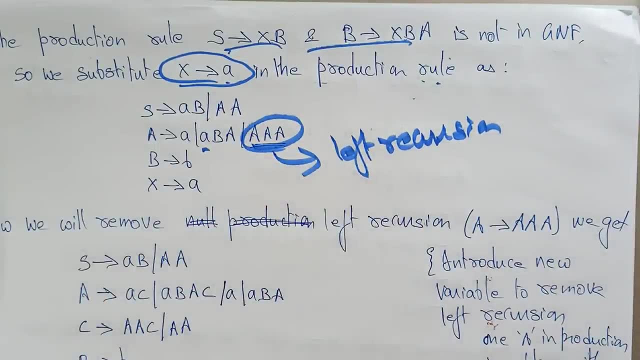 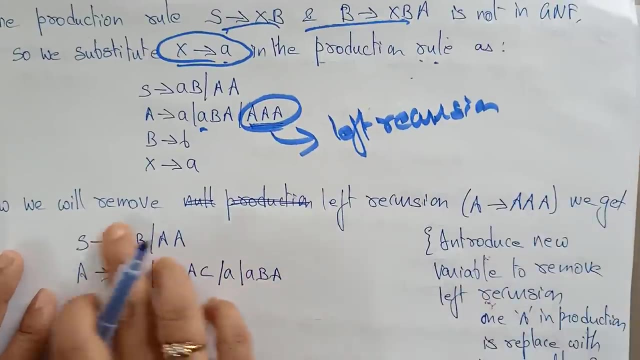 So there is no unit production. also is there? There is no epsilon productions, or is there? There is no? useless productions are also not there, Means the extra unused product terminal, non-terminals are also not there. Only the left recursion is there. Now we will remove this left recursion. 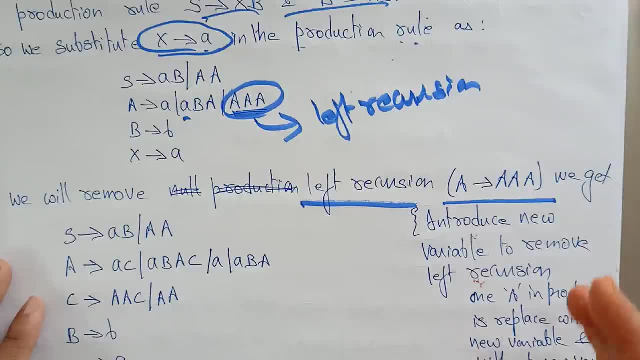 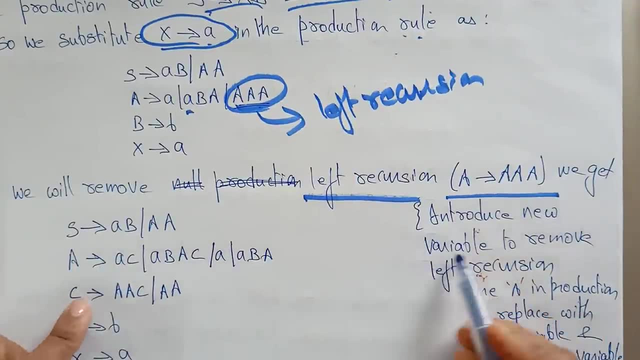 That is A, determine AAA. I have to be removed. How I can remove? What is the left recursion? What you are going to do, Just recall that, Introducing a new variable, I want to introduce one new variable C, to remove this left recursion. So what I am doing here, I am. 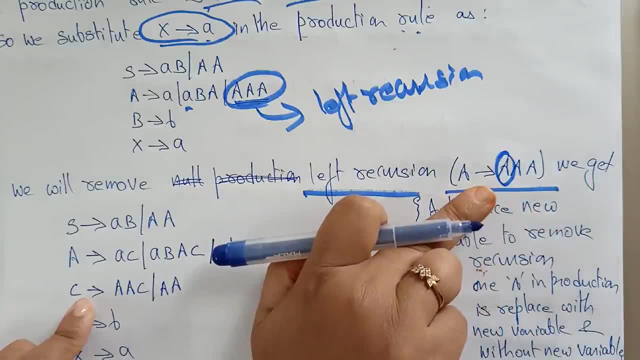 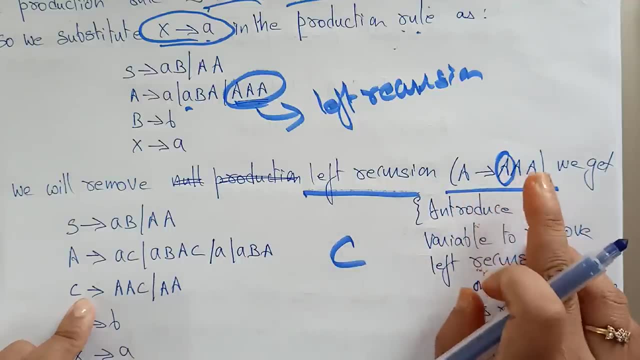 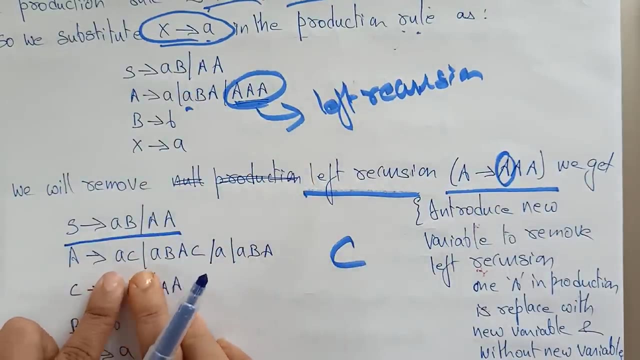 replacing one of this A, One. A in the production is replaced with a new variable and without new variable. So replace A with new variable and without new variable. Now let us see how it is. The first step is the same and coming to the step, second step: So this is A: A production. 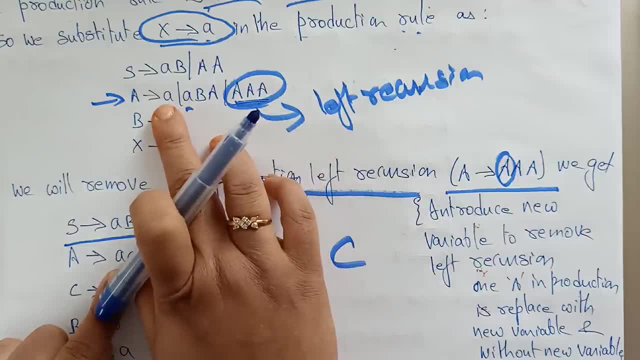 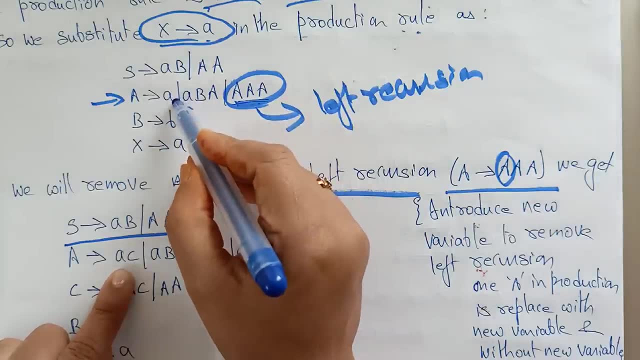 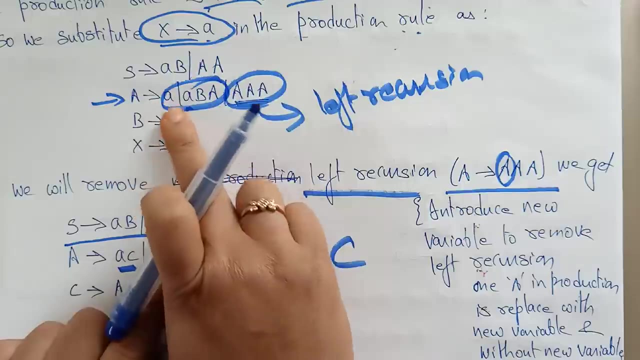 In this A production, the left recursion is there. Now I want to replace these productions with new symbol C as well as without new symbol. So with symbol C, AC, ABAC. So with A AC, ABC. Without new symbol: A, ABA. So this production. 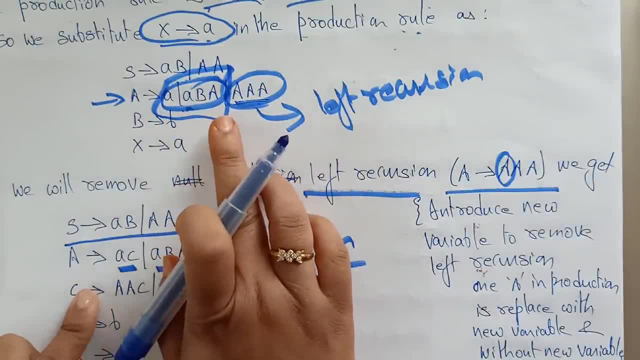 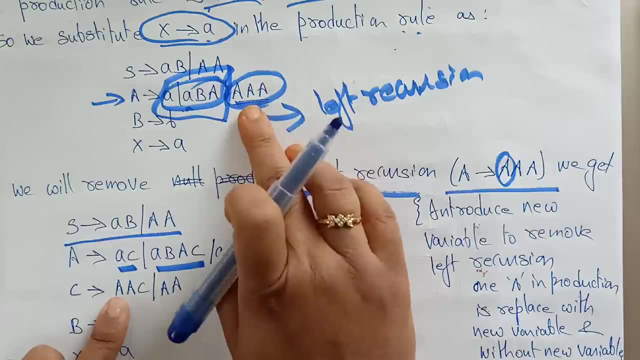 I have written like this: Only A determines A. slash ABA. I have written like: with new symbol and without new symbol. Now coming to this production. Okay, So this production. I already introduced a new variable, C, That is, C determines AA. 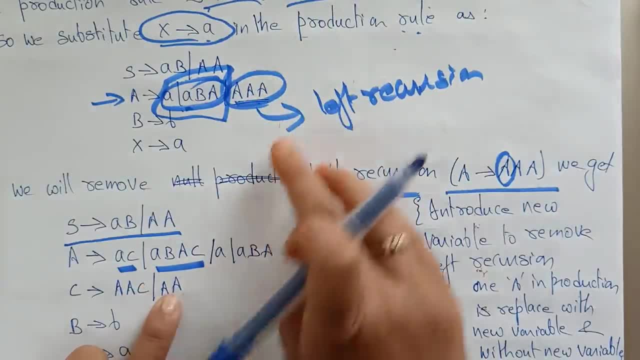 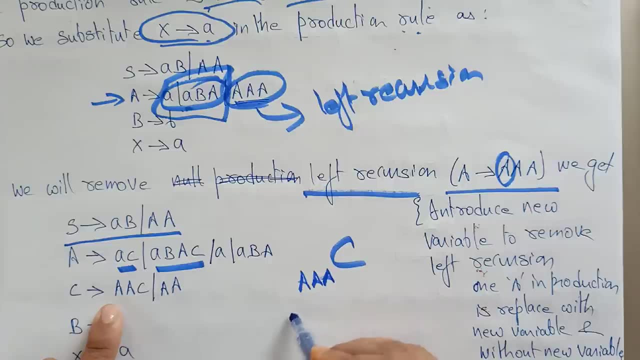 This A should be replaced with new production C as new symbol C and without new symbol, Without new symbol and new symbol. So this AA I replaced with a new production C with new symbol In place of single A. I added a new symbol and without new symbol. 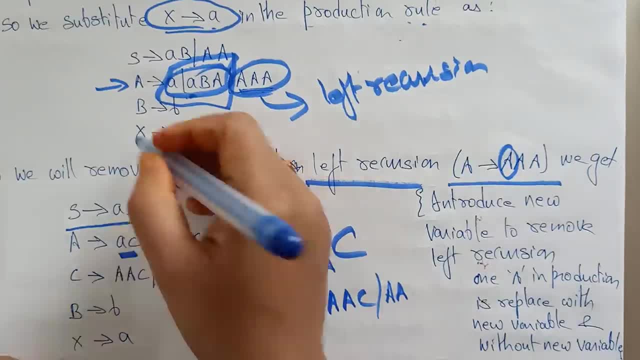 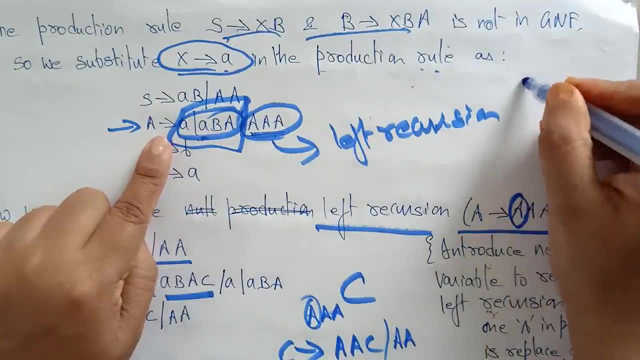 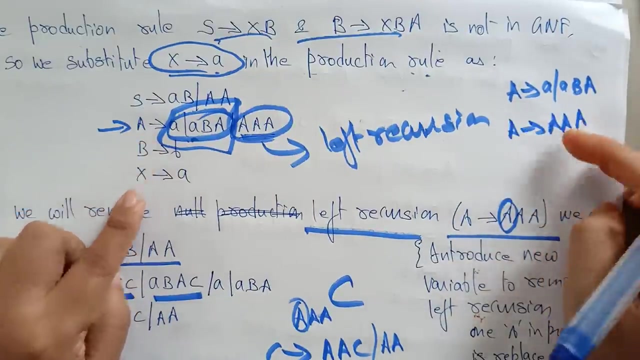 Okay, So this is how the left recursion can be done And BB and XB, XA or the C, Don't confuse. I just divided this into two productions. First, A: A slash ABA and A determines AA. So this having A has the left recursion. 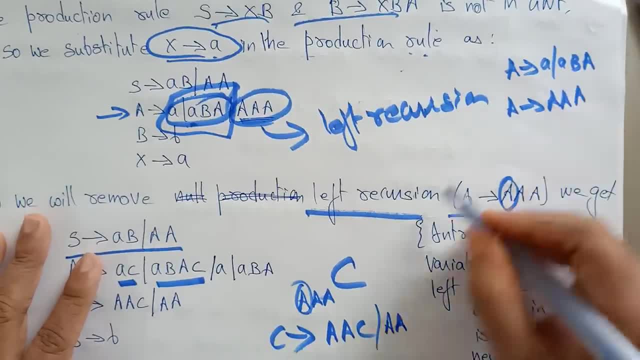 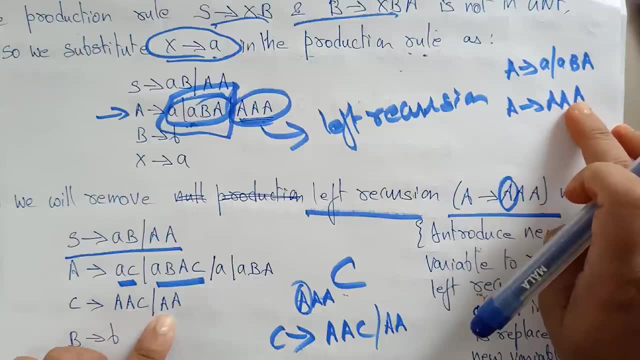 So I am just introducing a new variable C, That is, C determines with new product. A is replacing with new productions. new symbol C and without new symbol. Okay, So in place of here, also with new symbol, I have written this- and without new symbol. 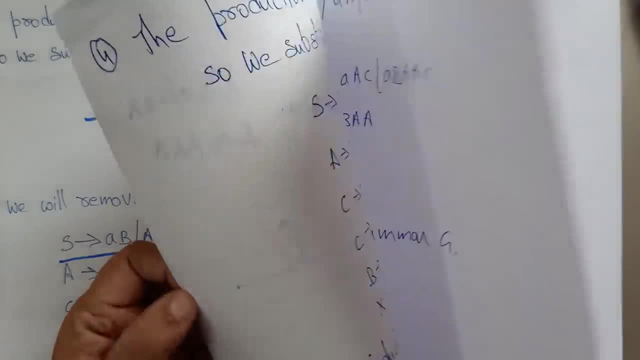 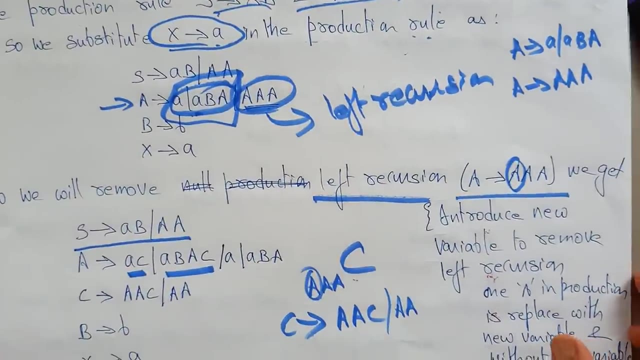 I have written this, Okay. So now the left recursion is also eliminated. Again, check The production rule. Check whether this is after removing the left recursion. is it is in GNF or not? Like check: This is in GNF. This is also in GNF. 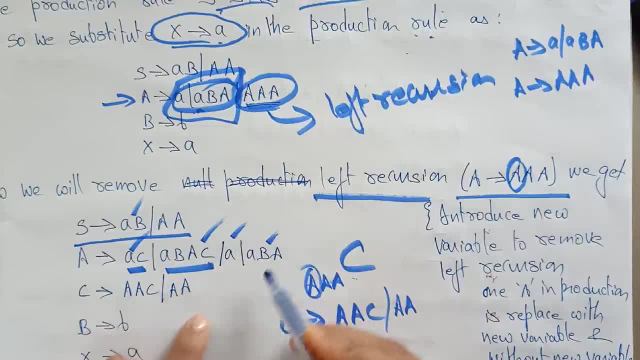 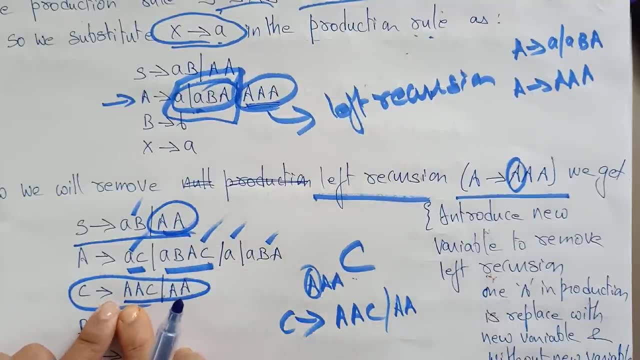 This is a terminal, followed with non-terminals: GNF, GNF, GNF. Okay, GNF, GNF, But only these are not in GNF, Because the start symbol should be here. The start symbol should be a terminal. 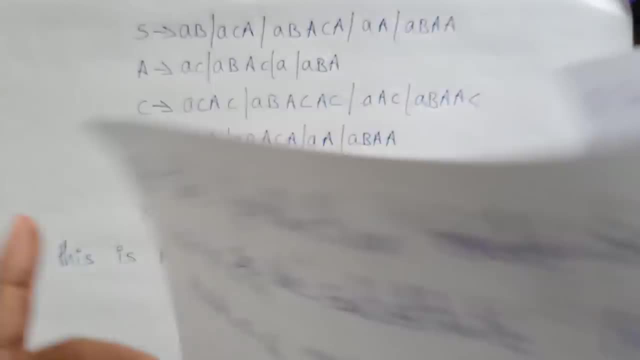 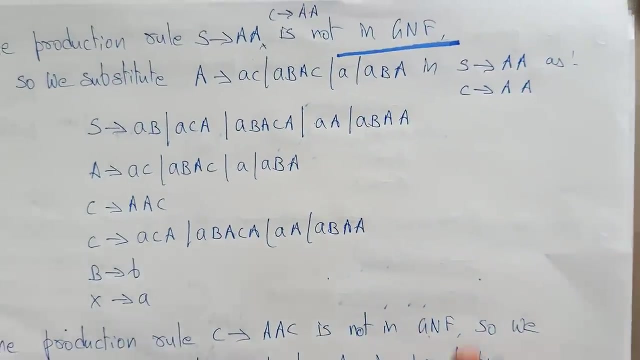 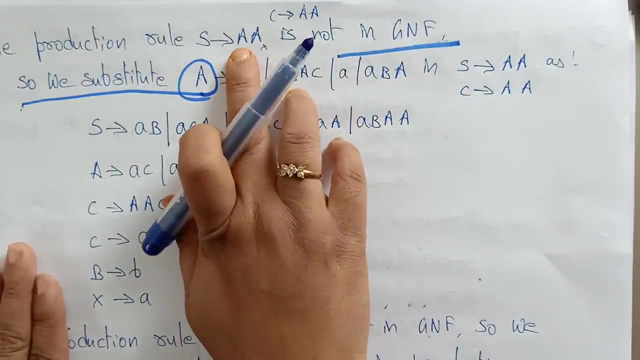 But there is no terminal here. Okay, So the production rules: S determines AA, C determines AA is not in GNF. So if those are not in GNF, what you have to do, You have to substitute Whatever the A production is there, that A production has to be substitute in these places. 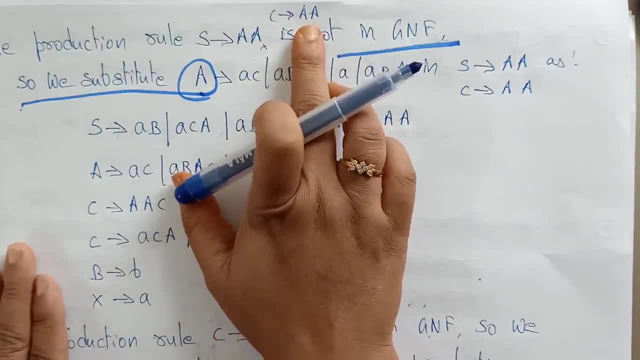 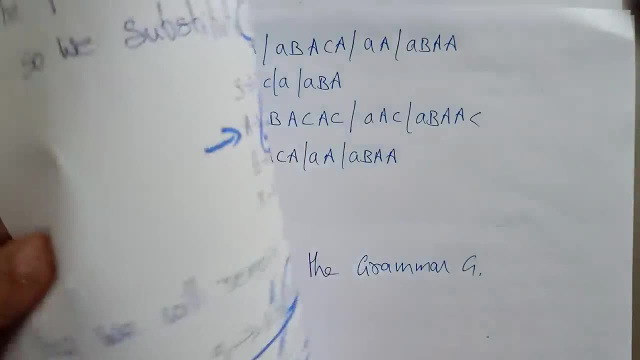 In place of S, determines A and in place of C, determines A. I have to substitute In one A In one A. I am substituting this: complete A production Here. already A production is there. Okay, I am substituting this A in one of the production. 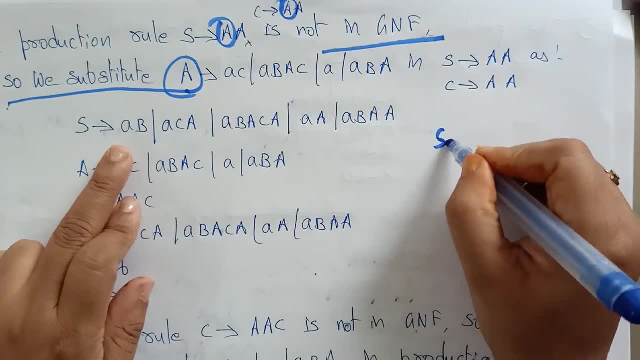 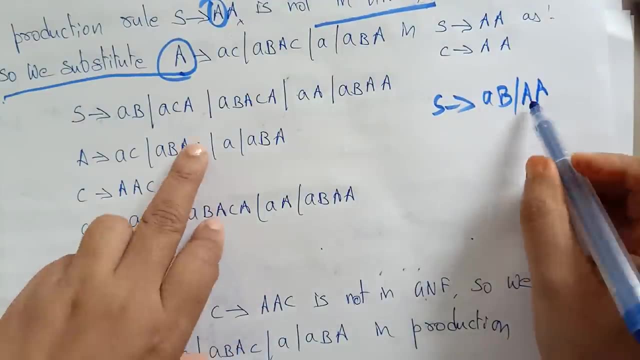 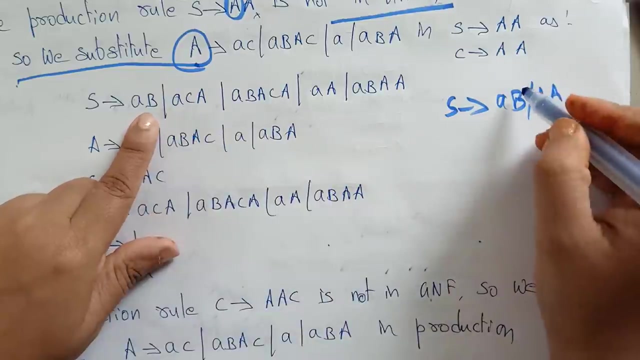 Now substitute. So what is actually? S determines, S determines ABA. So in place of one A, I need to substitute that production. So first is AB, AB, AB. I am writing as these. Okay, AB, I am writing as these. 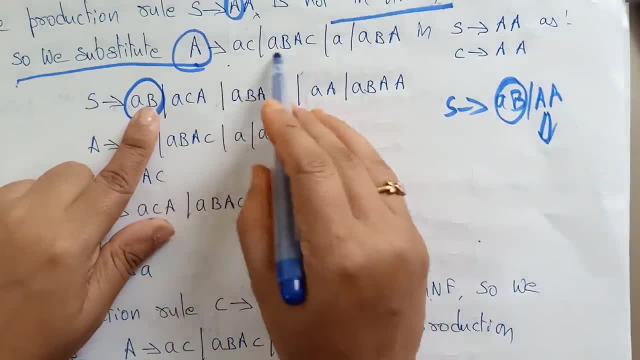 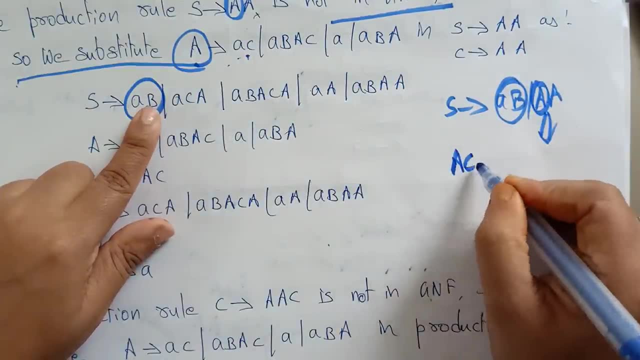 Now coming to this A, The first A. I am replacing this with production. So first AC. AC is multiplied with A. So in this A I am writing AC, A. Now coming to here. In this A, I am writing this production. 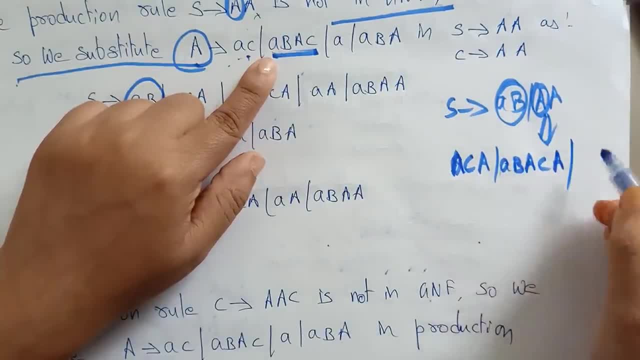 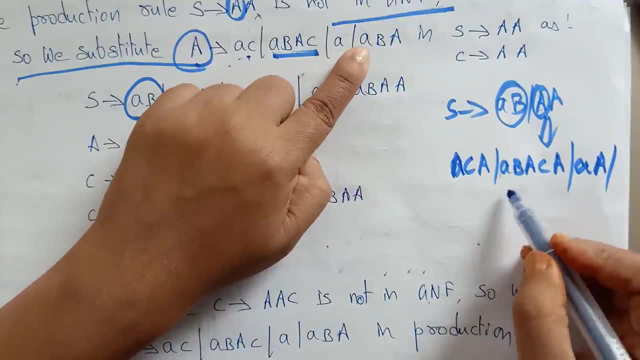 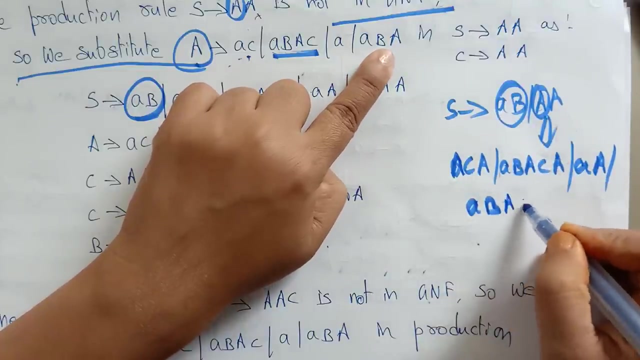 AB, AC and the remaining A you have to write here And coming to here In this A. I am writing this A along with this A. Now here, AB In this A. I am replacing with this production: AA, Okay, AB, A A. 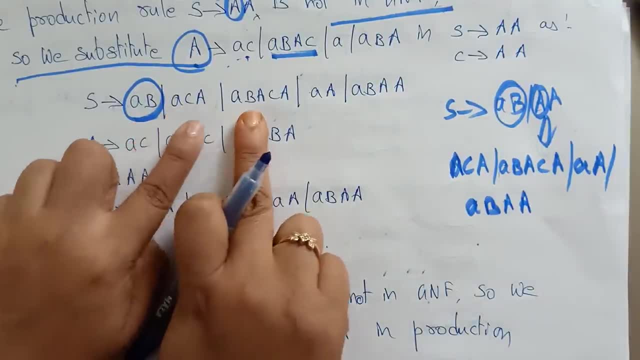 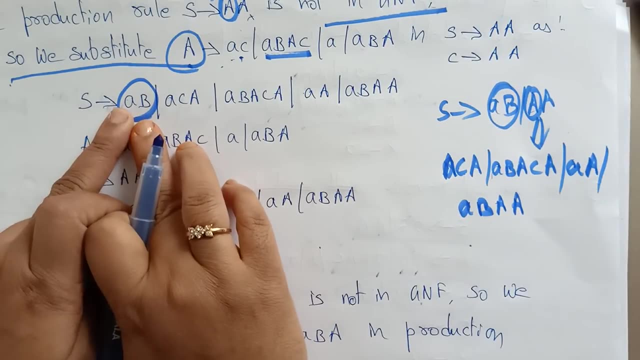 So this is what I have written here: AC A, AB, AC A, AA, AB, AA. I hope you understand AB as these I have written Okay, In place of one A, I am replacing this complete production. 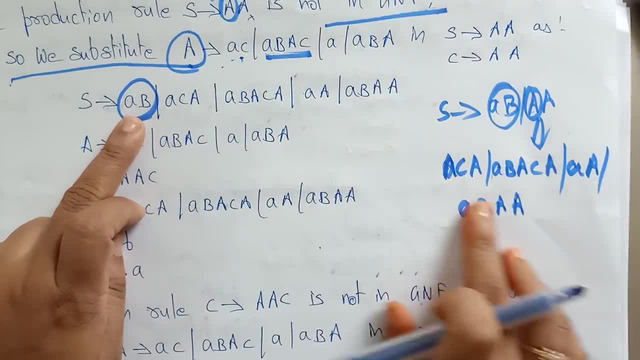 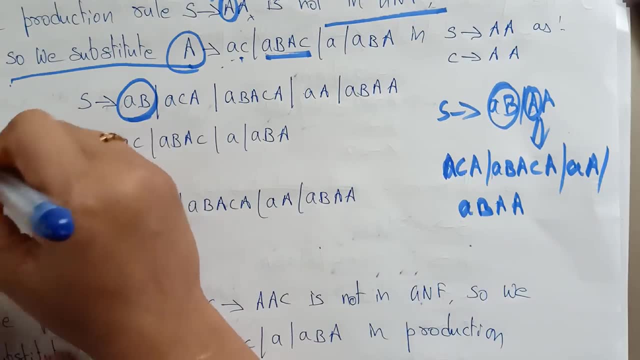 Okay, So for each production the remaining A has to be multiplied And that I have to return. So A is as it is Now. coming to C. C has two productions. So what are the? C has two productions. 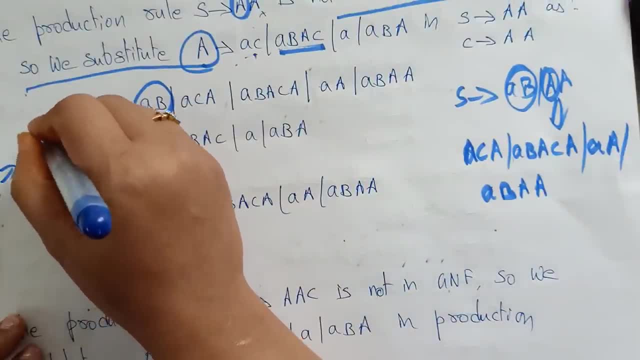 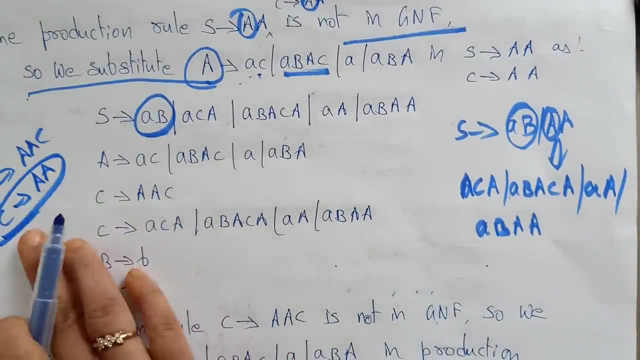 AAC and AA. AAC and C determines AA. So these two has a problem. So first thing is First- I am just concentrating only on this- I have written C, triple AAC like that. Later I will do somewhat substitution there. 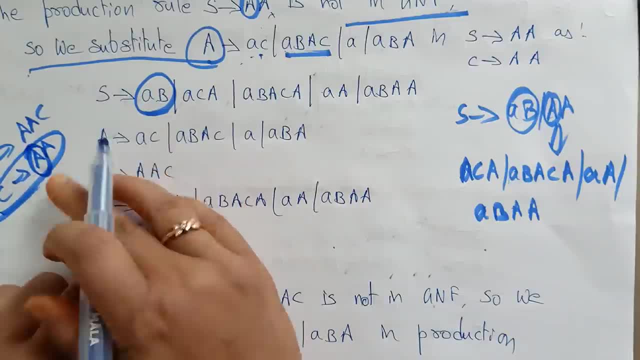 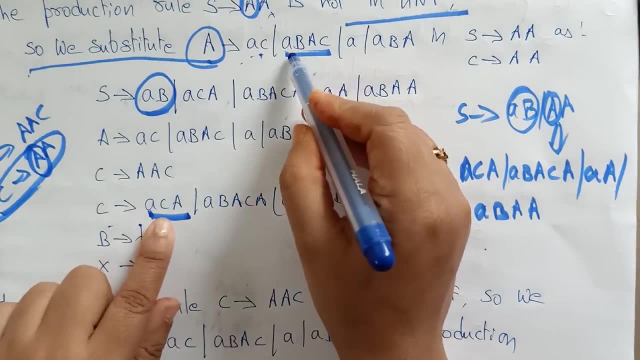 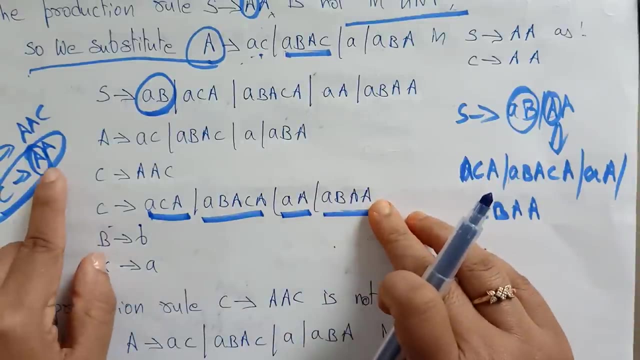 Now, coming to this C. C determines: in one single A I need to replace this entire production. So multiply this A with all these productions. So ACA, ABAC, CA and AA, ABAA. Okay, In place of A- one single A, I replace with this: 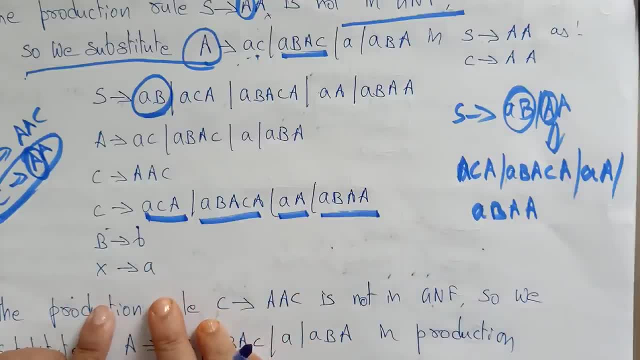 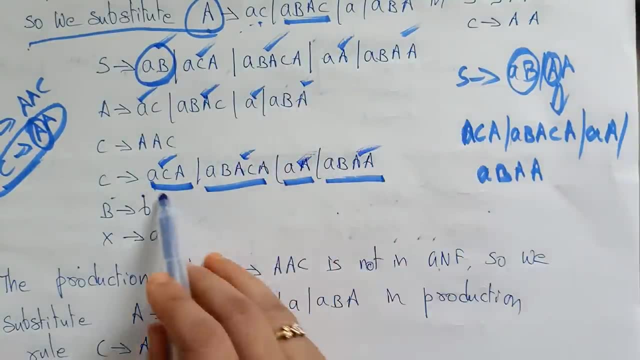 This is my C new production, B as it is, X as it is Okay. Now, coming to this: Everything is in GNF. Everything is in GNF Because a terminal is followed with non-terminals, But only these. It is in, not in GNF. 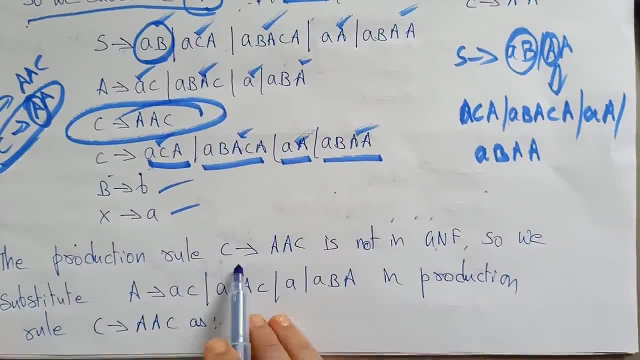 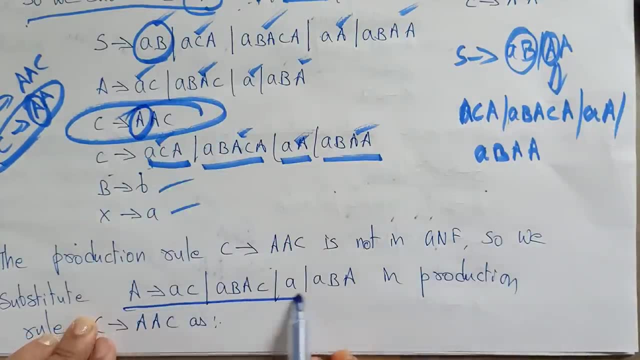 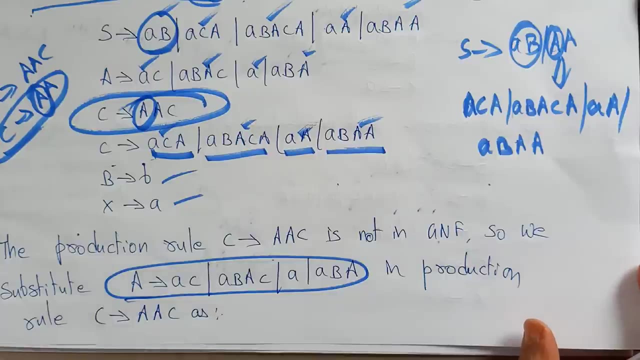 Because it is not following with the terminal. Now the production rule C determines AAC is not in GNF, So we substitute Here. also you need to substitute the A production. Now I, if you want, you can directly substitute here. I am to avoid the little confusion. 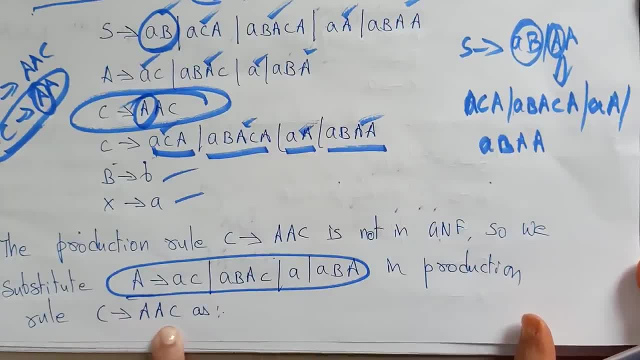 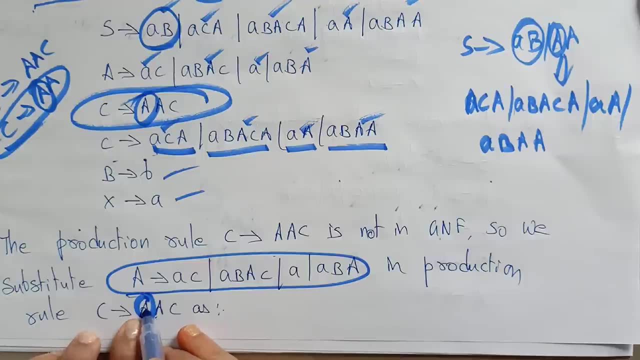 I am just substituting in another step. So C determines AAC In place of one single A, you substitute this. So if you substitute So in this A, you need to substitute this For how C determines In place of A first, this one. 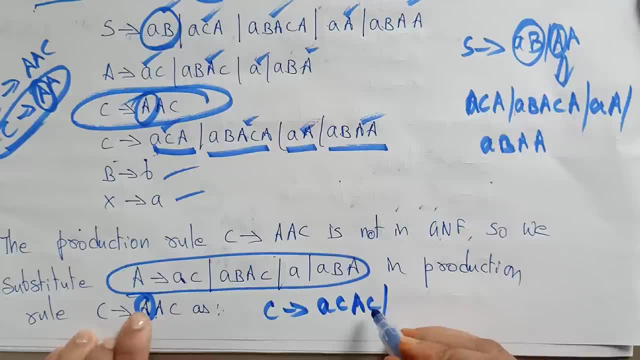 AC multiplied with capital AC. Next, in place of this, I substitute ABAC In place of A ABAC. The remaining two terms: AC you have to write. Next, in place of capital A, I need to substitute A.